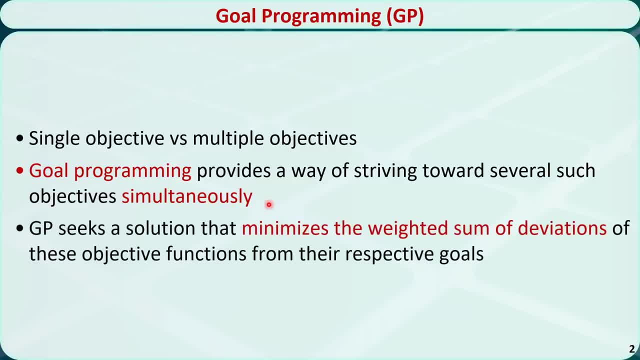 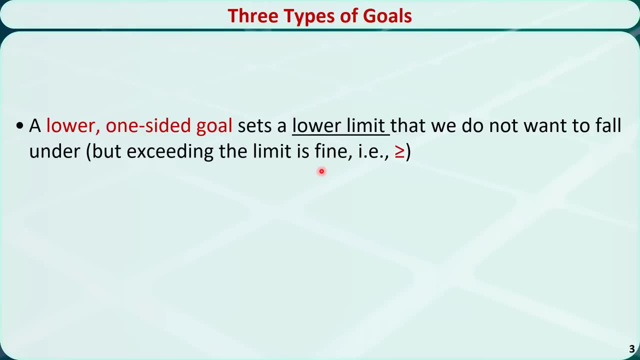 with such situations, It seeks a solution that minimizes the weighted sum of deviations of these objective functions from their respective goals. In general, there are three types of goals. A lower one-sided goal sets a lower limit that we do not want to fall under, but exceeding the limit is fine. This corresponds to a greater. 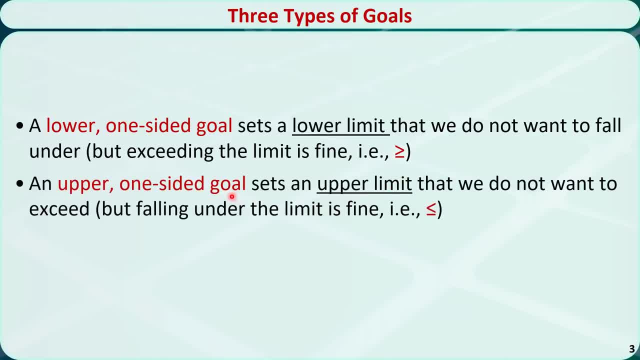 zone or equal to constraint. An upper one-sided goal sets an upper limit that we do not want to exceed, But falling under the limit is fine. This corresponds to a less than or equal to constraint. A two-sided goal sets a specific target that we do not want to miss on either side. This: 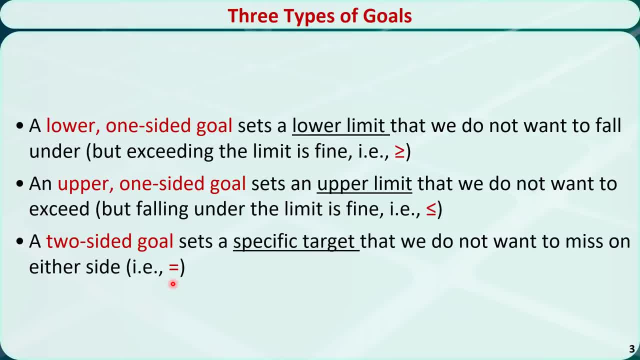 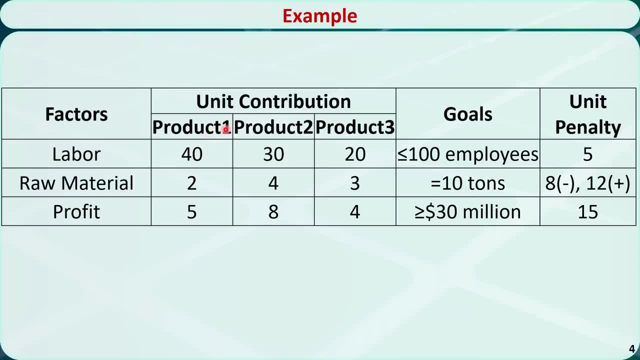 corresponds to an equality constraint. Let's see an example. A project manager is trying to determine the quantities of three types of products to produce. Producing one unit of product- one- we need 40 employees and 2 tons of raw material, and it will be. 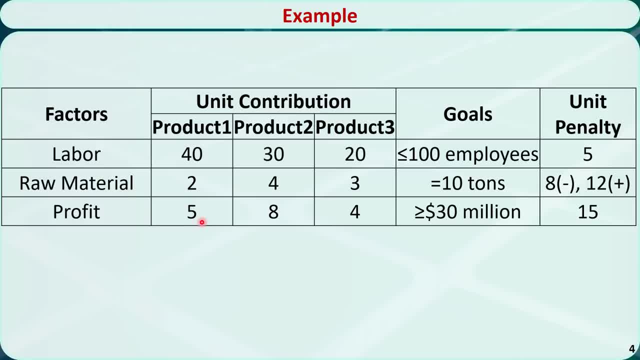 easy to bring the company $5 million of profit. For product 2,, these values are 30,, 4, and 8.. For product 3,, these values are 20,, 3, and 4.. The manager wants to meet these three. 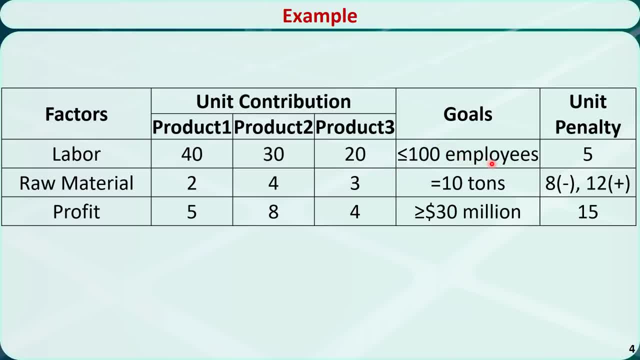 goals. First, the maximum number of employees that can be allocated to producing these products is 100.. Second, there are 10 tons of raw material in the warehouse. The manager wants to consume them all. No more and no less. The manager wants to consume them all. No more and no. 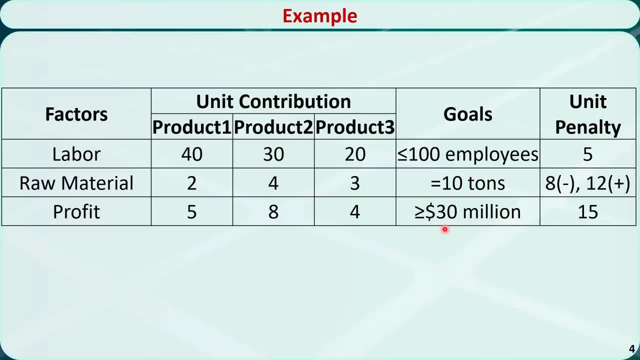 less. Third, the total profit is expected to be at least $30 million. The manager realized that it probably will not be able to attain all these goals simultaneously. Therefore, he sets some penalty weights for the unmet goals. If the project needs more than 100 employees, each extra employee is associated. 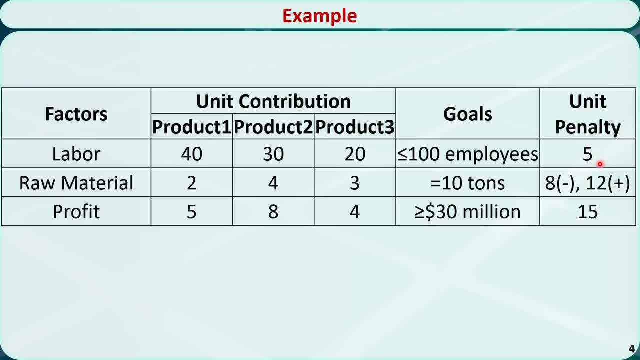 with a penalty of 5.. This penalty weight is unitless. If the total raw material needs is different from 10 tons, each ton that is below the goal is associated with a penalty of 8, and each ton that is above this goal is associated with a penalty of 12.. If the 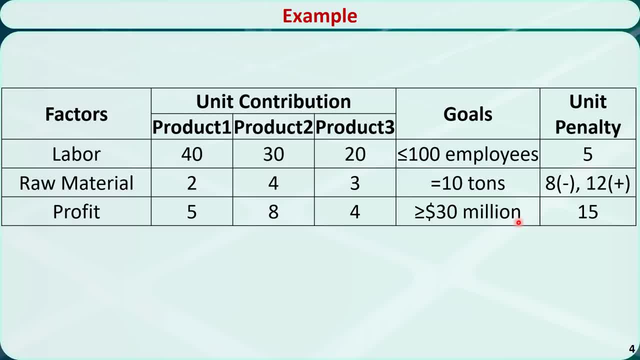 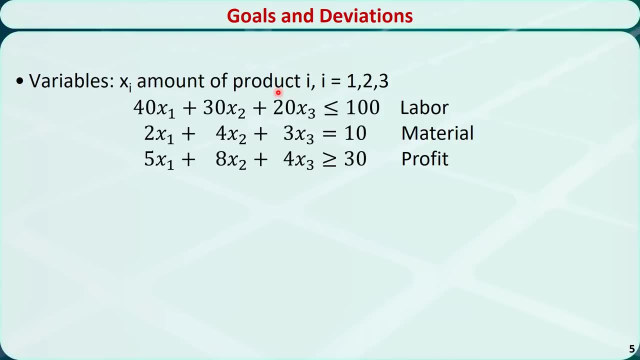 profit is less than $30 million. each million dollars under the goal is associated with a penalty of 15.. So the manager wants to minimize the total penalty. Let's define the decision variables. y is the amount of product i to be produced. i is equal to 1,, 2, and 3.. 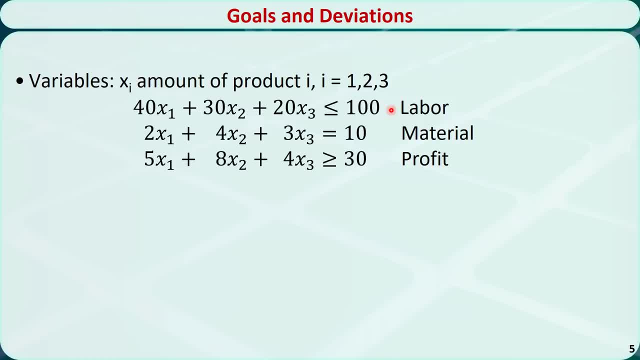 This is the first goal. The total number of employees needed should not exceed 100.. This is the second goal. The total amount of raw material should be exactly 10.. No more and no less. This is the third goal. The total profit should be at least $30 million. 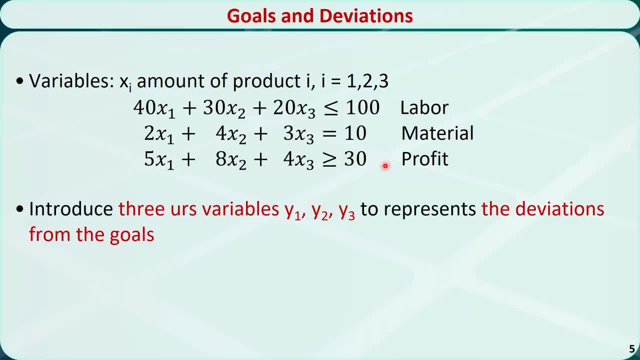 Now let's introduce three variables: y1, y2, and y3.. They represent the deviations from the goals. For example, y1 is equal to the number of employees needed in the project, minus the goal, which is the 100 employees If the needed. 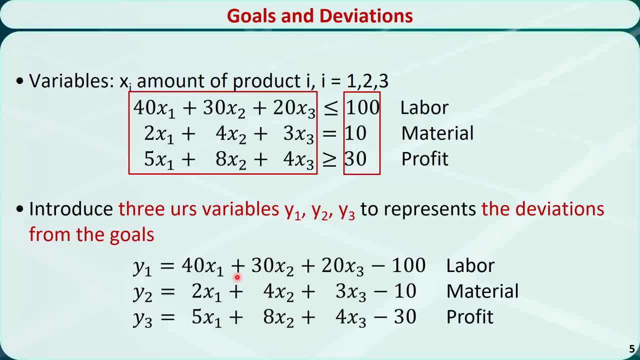 number of employees is less than 100, then y1 is a negative number. If the needed number of employees is equal to 100, y1 is 0.. If the needed number of employees is greater than 100, y1 is a positive number. Therefore, y1 is a negative number. Therefore, y1 is. 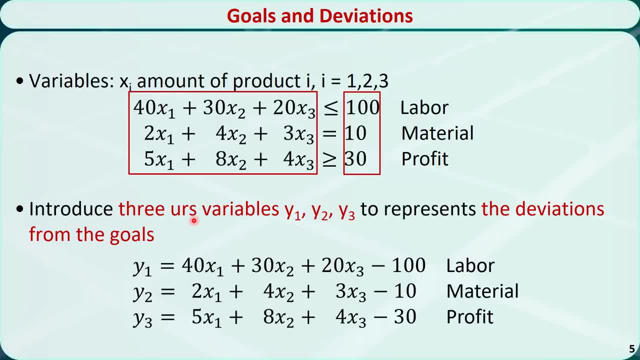 an unrestricted in sign variable, So are y2 and y3.. Now let me rewrite these three equations by moving some items to the left-hand side and others to the right-hand side. This is the new form We introduced in a previous video, that if we have an unrestricted in sign variable, we need to define two new variables to represent. 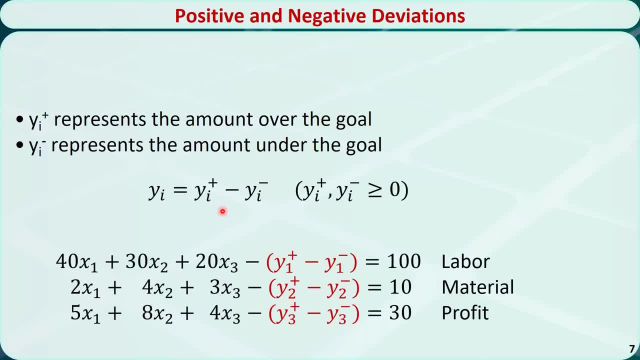 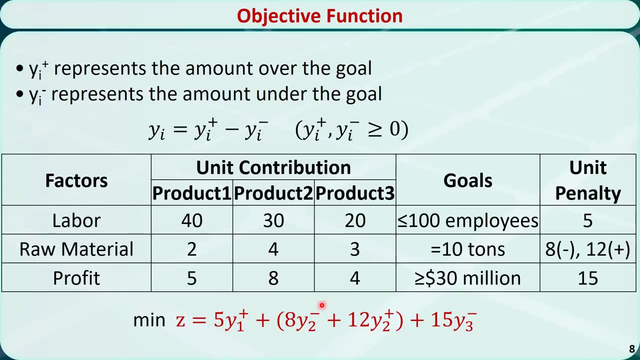 the positive deviation and the negative deviation from the goal and replace the unrestricted in sign variable with the positive deviation. Let's do that for these three equations. The manager wants to minimize the total penalty For the laborer. there will be a penalty only if the number of needed employees is over. 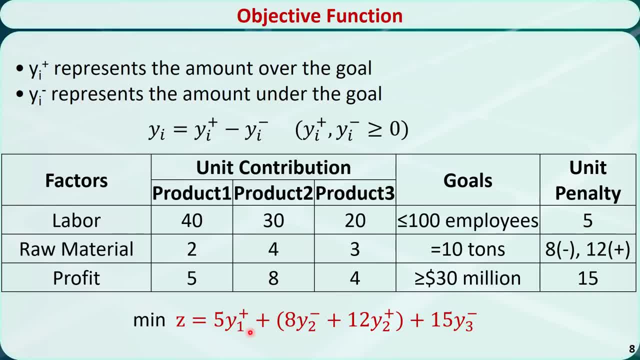 100.. So the penalty is 5 times y1+. For the raw material, there will be a penalty if it is less than 10 tons. There will also be a penalty if it is greater than 10 tons. So the penalty is 8 times y2-1.